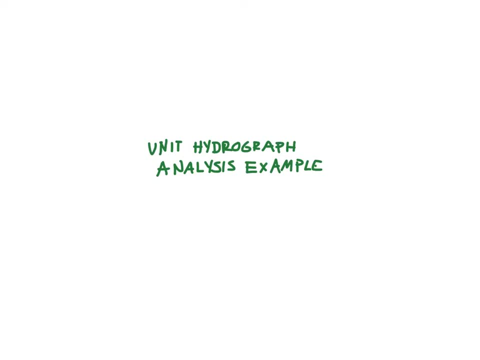 Hello. so in this video I am going to solve an example of determining a unit hydrograph. I'm going to go through all of the steps You can follow along with this example in the handout available on Camino in the Google Doc. 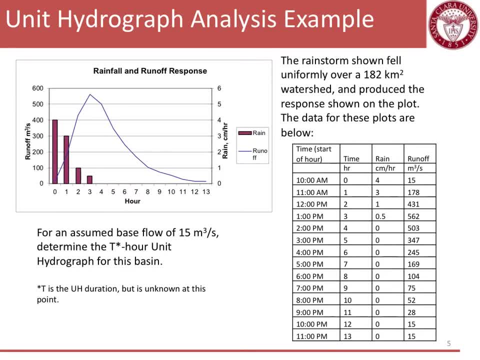 So here's the example: We have a rainstorm. It's shown as a bar chart on the figure, So you can see: the first hour, from zero to one, It rained four centimeters and then three centimeters, and then one centimeter, and then half a centimeter, And the rainstorm fell. 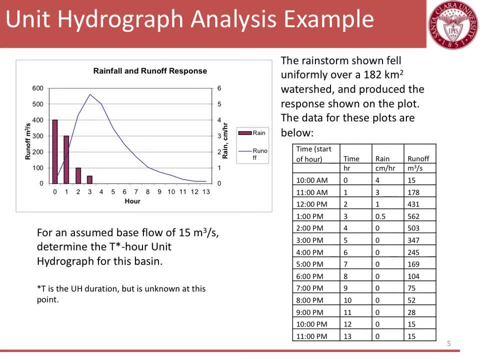 over 182 square kilometer watershed produced the response shown on the plot And we also have the data. We are going to assume a base flow of 15 cubic meters per second and we are going to determine the t hour unit hydrograph. 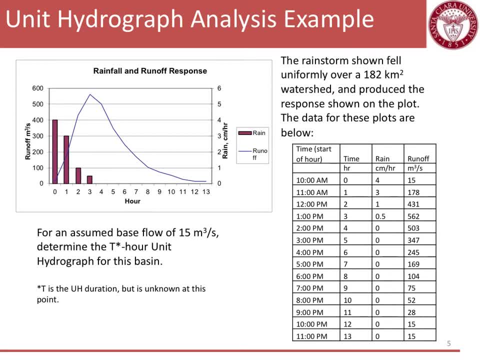 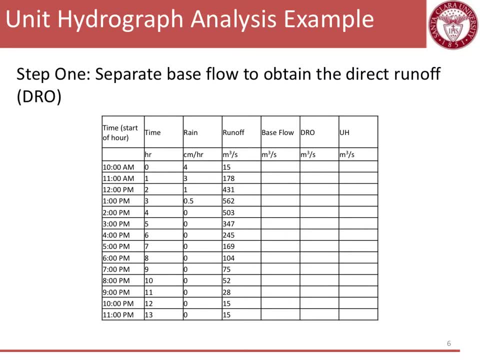 Okay, As part of this we will find that duration, but right now it's unknown. So our first step is to separate the base flow to determine the direct runoff. So in this case we were given in our problem statement what the base flow was. It's 15 cms, So we can go ahead. 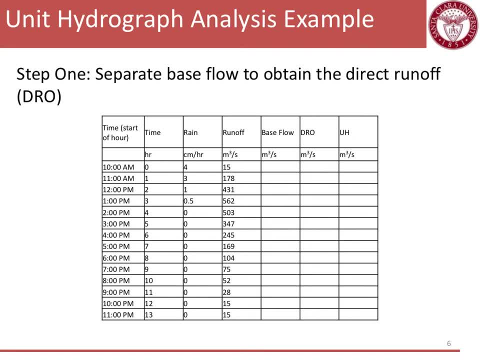 and fill in this chart quite easily. But there are other methods to estimate base flow, which I encourage you to look back in the textbooks and, on Camino, at the other videos and document I posted. In this case, we were told that the base flow was 15 cms, And so we can go ahead and 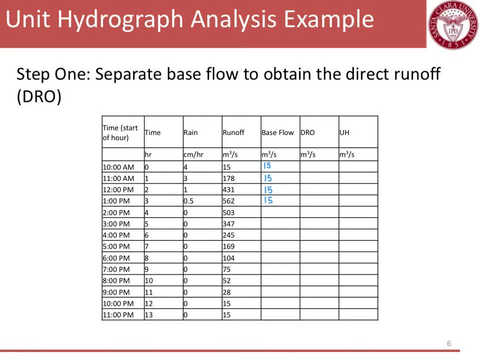 fill in this chart, this table, by just writing in, or you can see how easy this might be to do in Google Sheets or in Excel- And we're just going to put in the 15 cms base flow for the entire duration of the runoff. 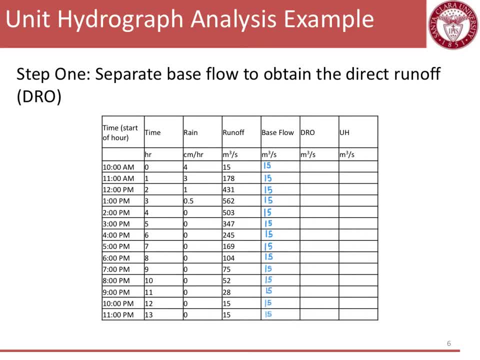 So to determine the direct runoff we take the runoff and subtract off the base flow. So this first time period at 10 am we had a runoff measured in the stream of 15 cms. We need to take out 15 cms for the direct runoff for the base flow, So we have a runoff. 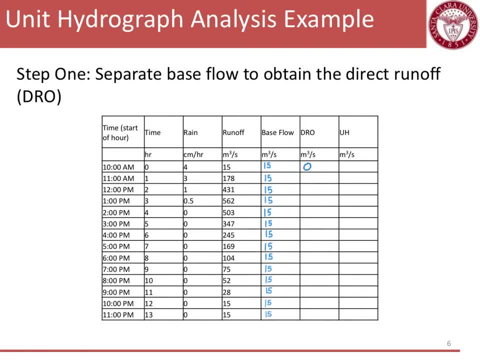 of zero. Okay, And in the second hour We have 15 cms. We have 15 cms, And then we have 15 cms for the second hour. So that's 178 observed, and so we're going to subtract out 15 and get 163 CMS. yes, I'm. 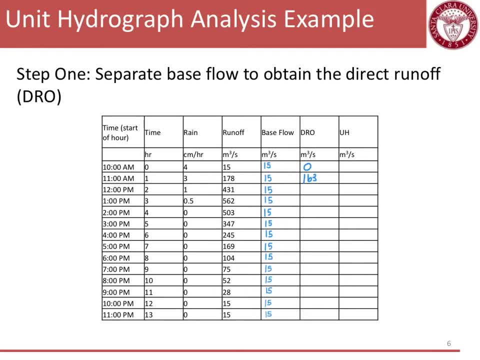 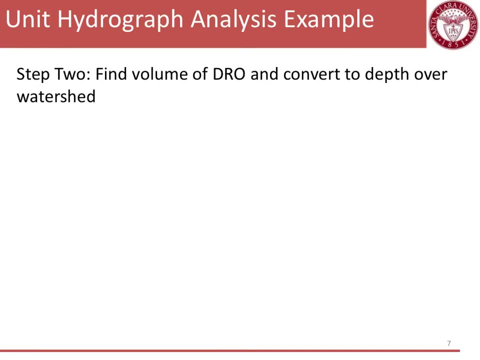 going to go ahead and fill in the rest of this table and encourage you to do the same. alright, so there is the direct runoff, which is just again the runoff minus the base flow, and we are now done with that first step and we can move on to the second step. and the second step is to find the volume of that direct. 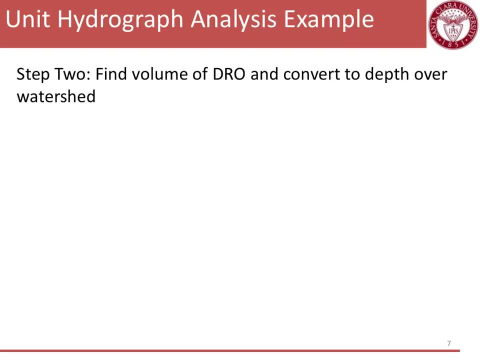 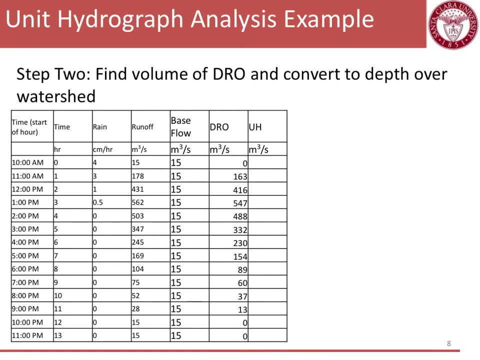 runoff and convert it to a depth over the watershed. and so the approach we are going to do to accomplish this is to take and sum up the direct runoff which will be in CMS, and I convert that to a depth, just like we've done many times for total rainfall. so if I took that in total, that total column of direct 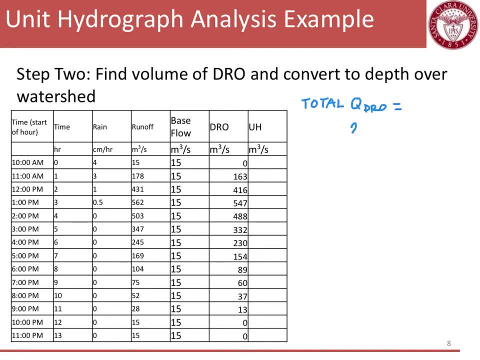 runoff and summed it all up, we would get a runoff of two thousand five hundred and twenty nine cubic meters per second. we would like to convert this to a total volume, and so I'm going to do this by taking that two thousand five hundred and twenty nine cubic meters per second and first. 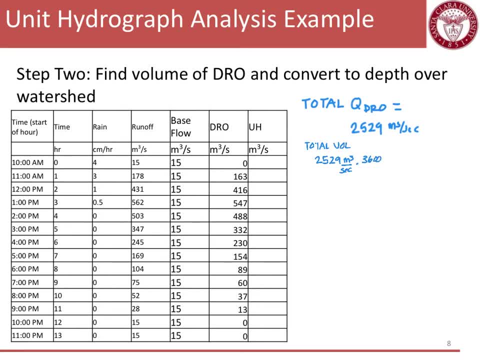 converting it into a time base of an hour. and so if you do this you will get nine one zero four four zero zero meters cubed. so I'm going to do a little mental manipulation math here and convert that to nine point one zero four four kilometers squared. 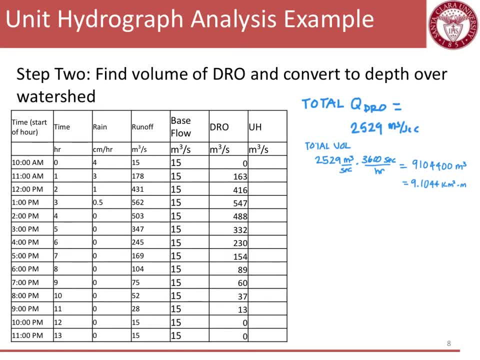 times meter, and I did that because my watershed area was given in square kilometers. so then I can easily convert this total runoff volume into a depth of rain by taking the nine point one zero four four kilometers squared per meter, dividing by that a hundred and eighty two. 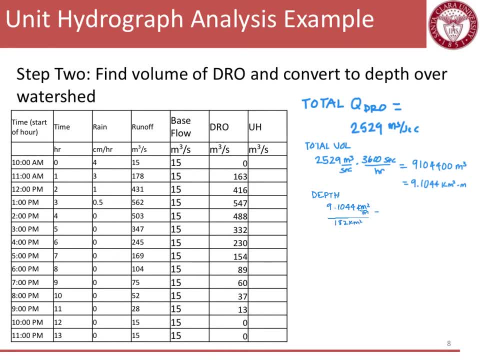 squared kilometers, which gives us a depth of zero point oh five. zero zero two four meters, which is five point O centimeters. isn't it amazing how that worked out to exactly five centimeters. it's just a miracle. so my rainstorm let to a depth of five centimeters of rain. 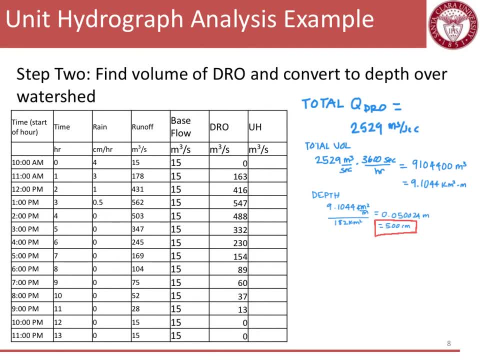 So this is a particular storm where I was able to measure the rainfall coming in and the storm runoff in a stream, a gauge stream coming out, And so to convert that to a unit hydrograph, what I want to do is make it represent a depth of one centimeter. 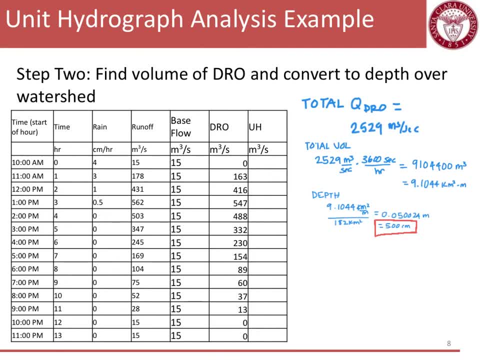 falling on the watershed, And so to get from five centimeters to one centimeter, what I need to do is I need to divide by five or multiply by one over five, right? So I am going to take each of my direct runoff. 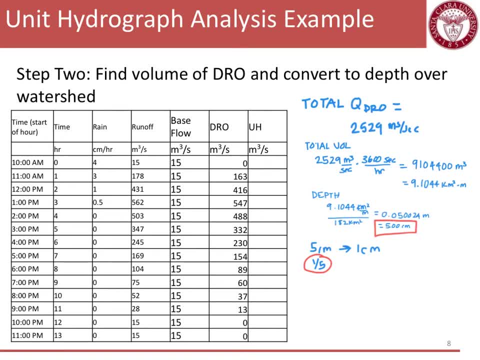 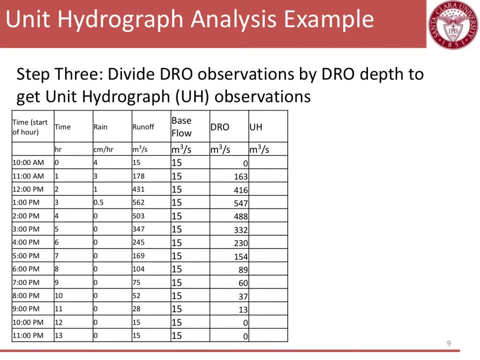 And the next step, I'm going to take each of my direct runoff values and divide it by five. Okay, so we're going to do that on this table. And again, just to repeat what I'm going to do, my direct runoff divided by five. 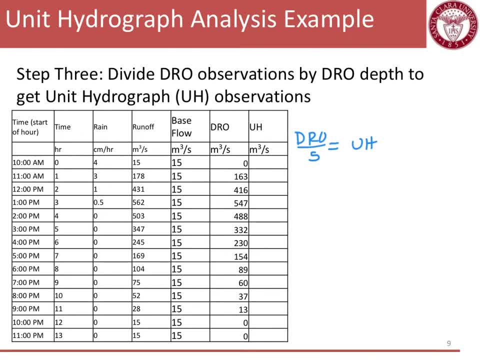 Is going to be equal to my unit hydrograph. So easy. first one: zero divided by five is zero. Okay, The next one, 163 divided by five, is going to be 32.6 cms. So I'm going to continue this for the entire table. 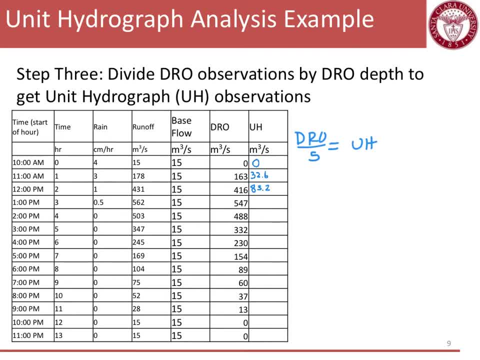 So my next entry is 83.2 cms, So I'm going to stop this. fill in the rest of the table And I encourage you to calculate these for yourself As well. Okay, so here's that table, filled in, And we can do a quick check to make sure that our numbers are right. 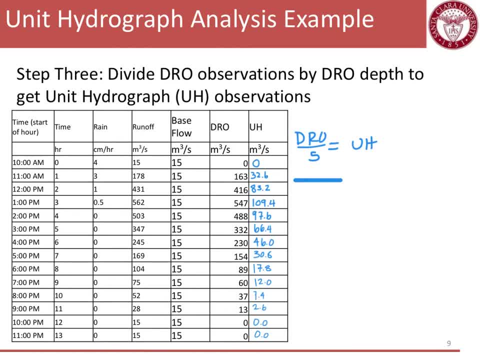 And the best way to do that is to actually kind of repeat what we did in the last step. Just take the sum of your unit hydrograph values. If you do that, you should get about 505.8 cubic meters per second. This gives a total. 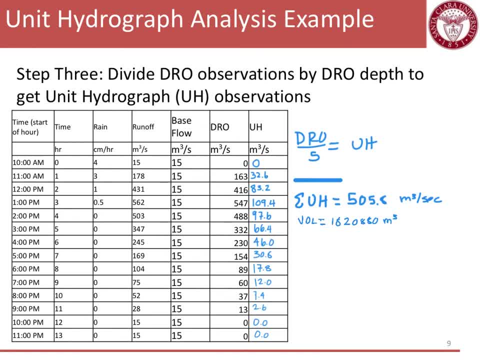 Volume over the watershed of 1820880 cubic meters, which is 1.81 kilometers squared per meter, Which, if you again divide by the area of the watershed, leads to one centimeter, which is exactly what we want, And now we have a unit of rainfall. 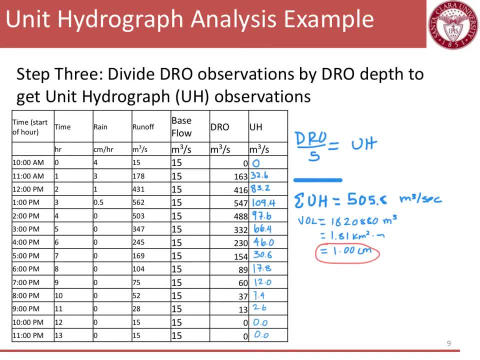 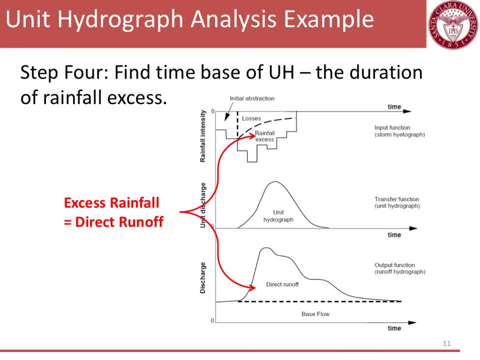 So we're close to it. We're right at that, You know we're right at that. unit hydrograph. All right, our last step: we want to find the time base of this unit hydrograph. We want the duration. Okay, so right now it's just we call it a T star, but we want to figure out that duration. 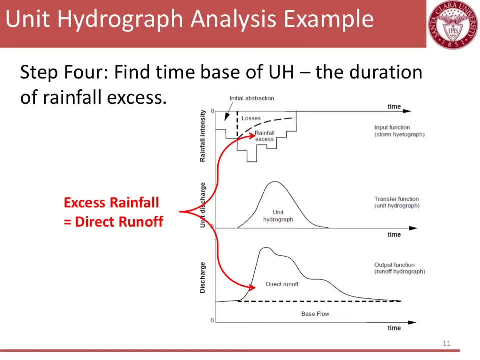 And so we have to figure out how long we had rainfall excess. Okay, so we want that unit of rainfall, that one centimeter. We want to see how long it took to get that one centimeter, Once we take away all of the infiltration and other abstractions and losses. 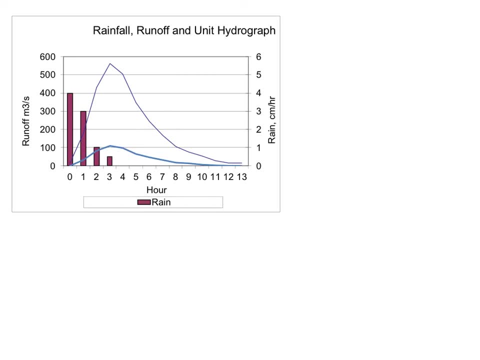 And so to do that, we're going to take a close look at that hydrograph, which is shown in the by the purple bar charts here, And so from this, we had first four centimeters of rain, then three, then one centimeter rain and then 0.5 centimeter of rain, each of those for one hour. 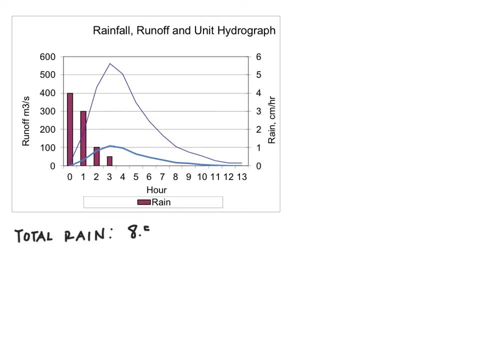 So our total rain here was 8.5 centimeters of rain. We know from our Previous steps that the total runoff that we observed from this storm was five centimeters. So that means that in the four hours we had a loss of 3.5 centimeters of water. 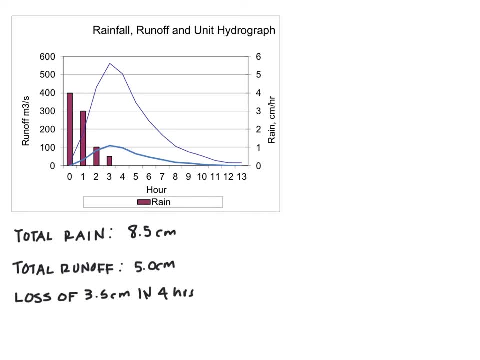 In those four hours. Okay, So, just like we did when we first started talking about infiltration, we're going to use the fee method here And just try and guess, So that three and a half centimeters in four hours is 0.75 centimeters per hour. 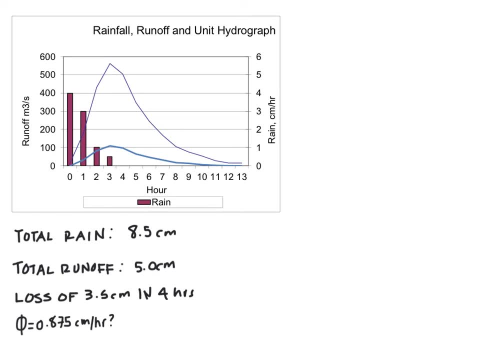 So if we use that as a fee or a loss, does that lead us to five centimeters total runoff? Let's look at a table of data to figure that out. All right, So I have this table where I'm going to show the time, which is an hour, from, for example, zero to one. 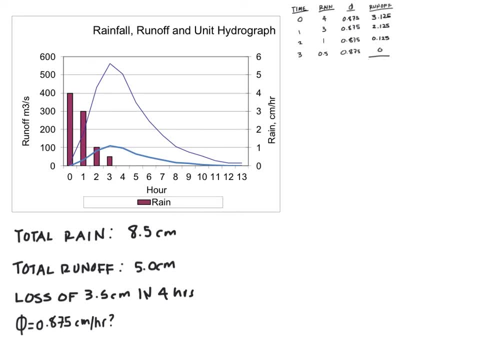 The rainfall in centimeters per hour, the fee and then the runoff. Okay, So in that first hour from zero to one, we had four centimeters of rain. We're estimating a loss of 0.75 centimeters per hour, leading to a runoff of 3.125.. 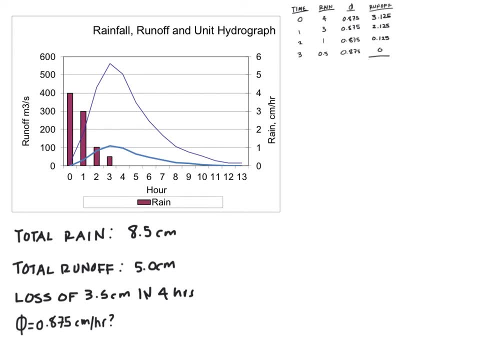 All right. So remember in that last hour that three to four we had less rain than the amount that could infiltrate, So we had no runoff. If we sum up all these runoffs we will get a total, A total of 5.7, 5.375 centimeters of runoff. 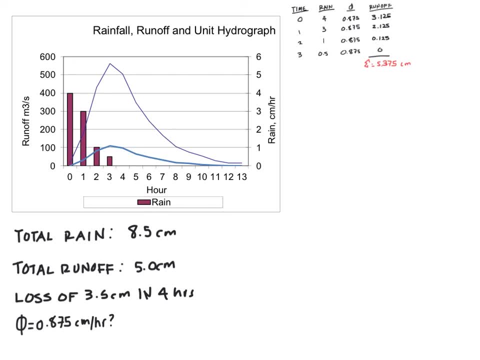 This is greater than what we observed- the five centimeters- So our fee needs to be a little bit bigger. Okay, So let's try a new fee, Let's try a fee of one and see what happens. So now I've assumed a fee of one centimeters per hour, which now I'm showing the runoff again here on the right hand side. 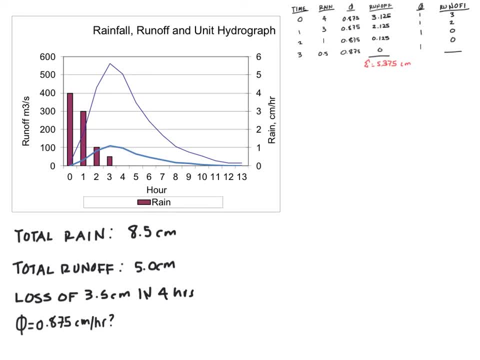 In that first hour I'll have three centimeters, The second hour two centimeters, And then in the second and third hour, no runoff. And you can see here that now my sum of the rainfall that becomes runoff is five centimeters. 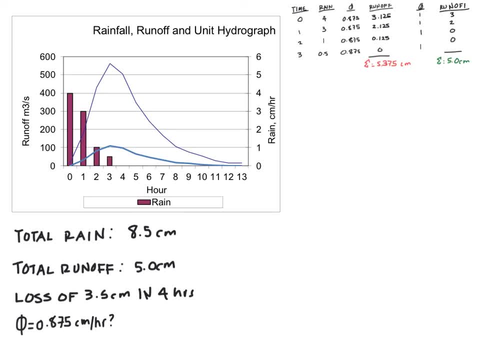 which matches what I observed in the stream flow. So this suggests that the rainfall excess occurred in two hours. Okay, So that rainfall excess occurred in two hours, which means that this unit has a runoff of 0.25.. Okay, So that rainfall excess occurred in two hours, which means that this unit has a runoff of 0.25. 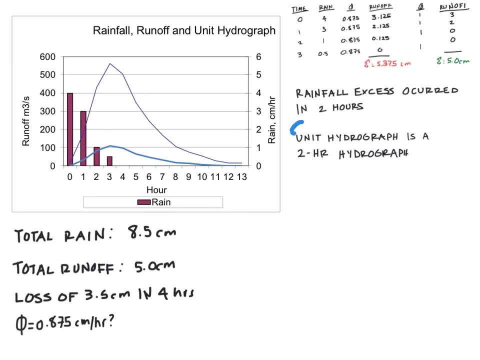 And we can see here that the two hour unit hydrograph is a two hour hydrograph. Okay, So if we go back to that problem statement, we would call this a two hour unit hydrograph. And this becomes really important when we apply the unit hydrograph to different storms. 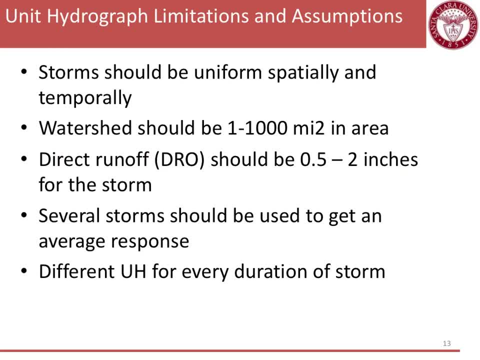 All right, So that's the end of the example. I just wanted to talk about a few limitations in using unit hydrographs. So the first one is that storm should be uniformly- should be uniform both spatially and temporally. OK, so maybe a pretty uniform rainfall, and that uniform rainfall needs to be spread evenly through the throughout the watershed. 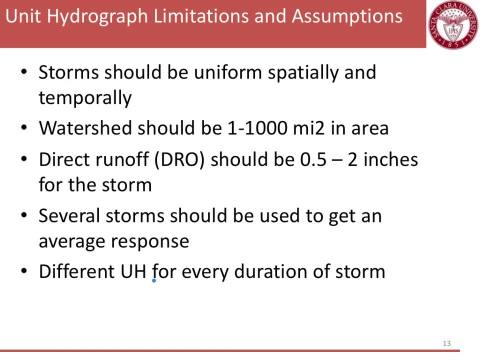 The watershed should be between one and 100 square miles in area. OK, so not too big and also not too small. Too small, I'll just use the rational method. The direct runoff should be point five to two inches for the storm. 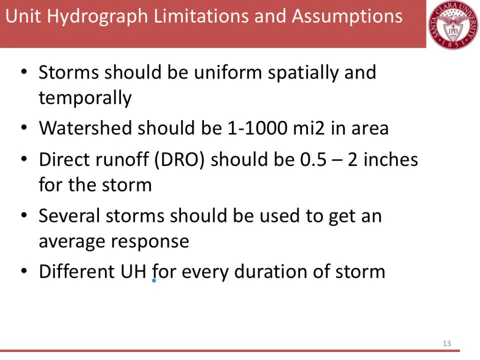 And when you're actually creating these, you know hydrographs. you want to use several storms to get an average response And you also need a different unit hydrograph for every duration storm, And we will talk about that moving forward as well. All right, 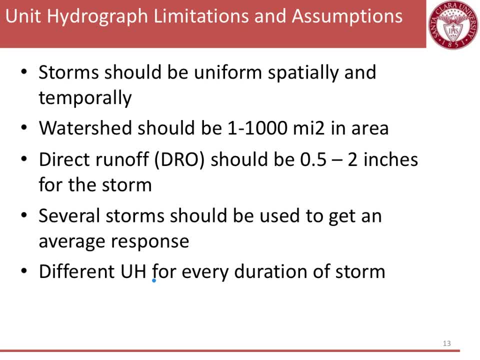 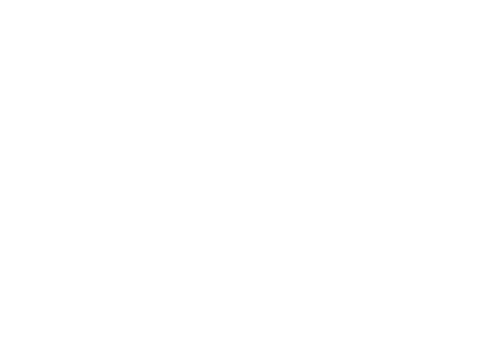 So that's the end of this. I'll do some a bigger problem solving session in a live Zoom later this week. Thank you, 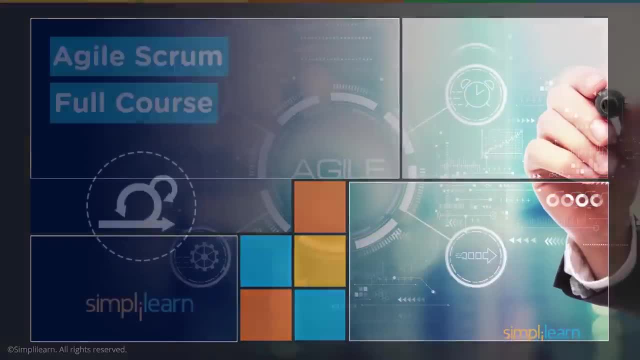 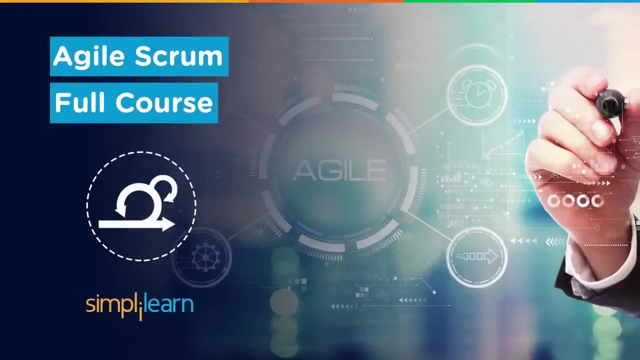 Hello everyone, Welcome to this Agile and Scrum full course by SimpliLearn. In this session, we will tell you everything you need to know to become well-versed in the concepts of Scrum and Agile in less than 4 hours. Our instructors, Chandra, Rahul and Ishan, will be covering topics 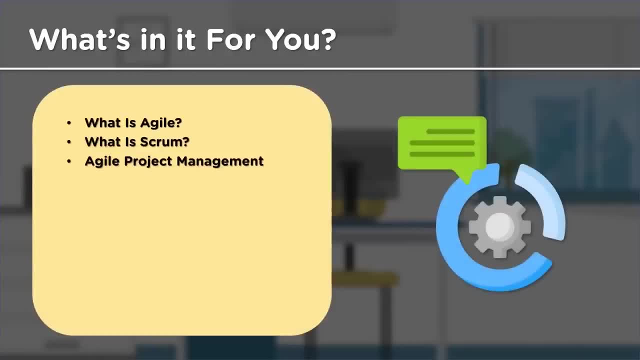 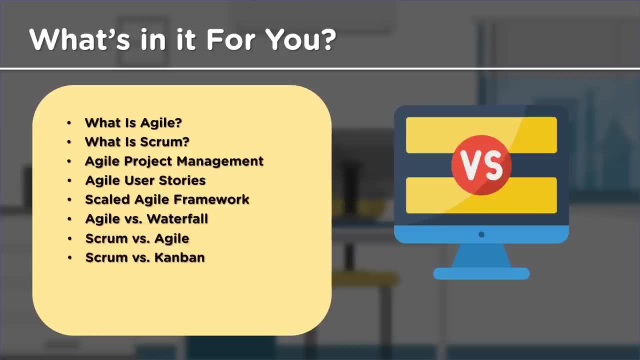 like Agile Scrum, Agile Project Management, Agile User Stories, Scaled Agile Framework, how Agile Waterfall, Scrum and Kanban are different from one another, and many more. We will also be guiding you on how you can become a Scrum Master. We will be learning. 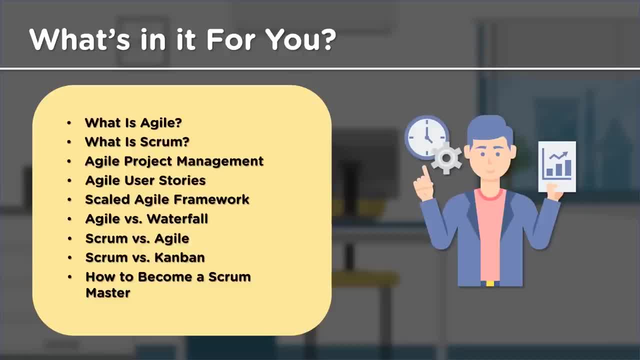 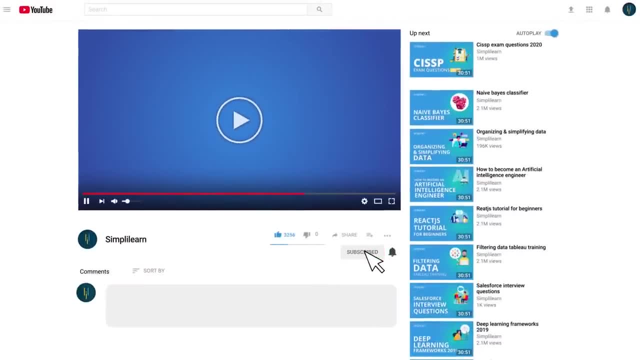 all of this in under 4 hours, So without any further ado, let's get started. But before we begin, make sure you have subscribed to our YouTube channel and don't forget to click on the bell icon so you never miss an update from SimpliLearn. 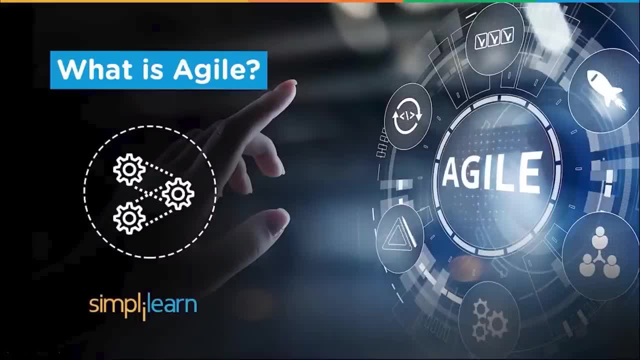 Welcome to Agile tutorial from SimpliLearn. I am CMR Chandra MR, a Professional Consultant and Coach, Certified Agile Scrum Master, PMP, Prince2 Practitioner, ITL4, Managing Professional COBIT5 and DevOps. As part of this video tutorial, we are going to understand what is Agile.